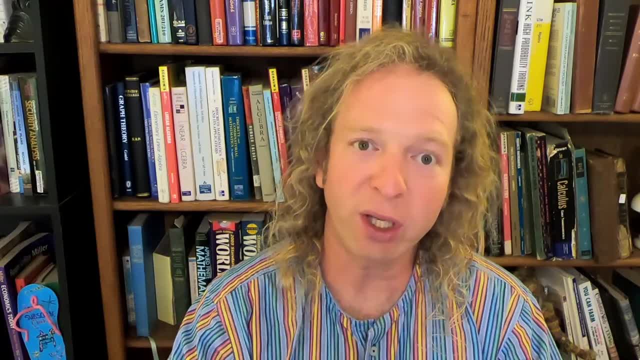 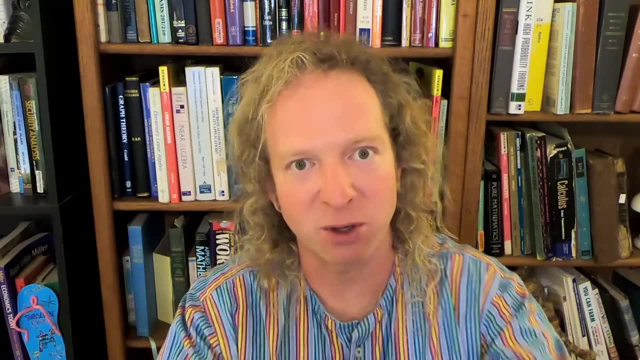 even or y. I was fortunate enough to have some really, really good teachers during my undergraduate education. that helped me learn how to write proofs, because they would grade my work And they would give it back And they would mark stuff wrong And in class. 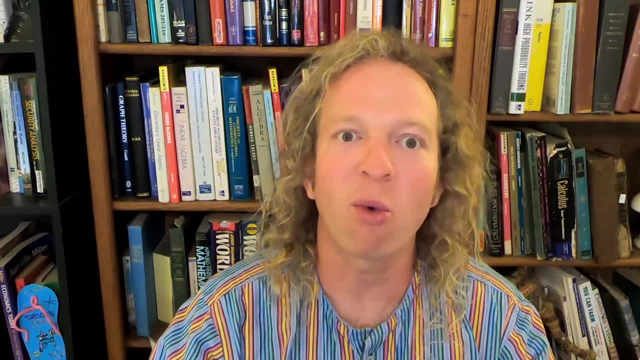 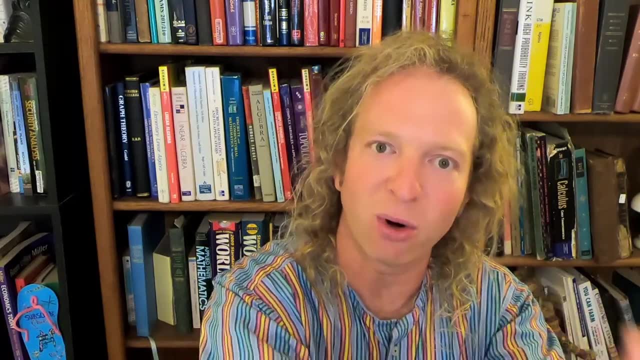 they would show all of the steps. So that's the key: You need someone to show you all of the steps, And then what you want to do next is you want to mimic that. You want to mimic someone else's work. Show the steps like they do, So find. 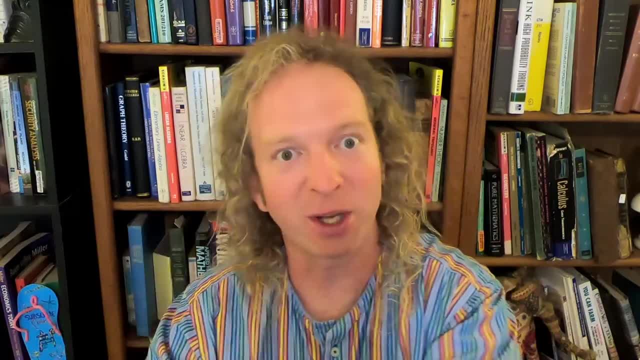 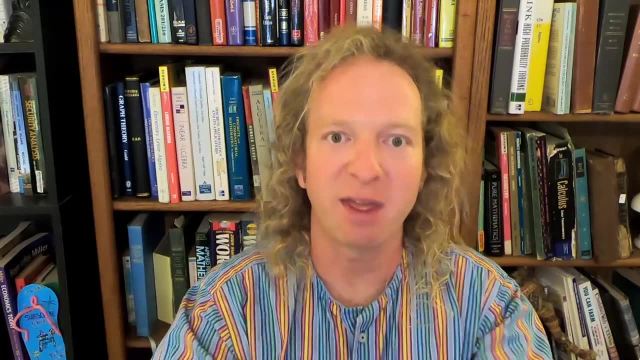 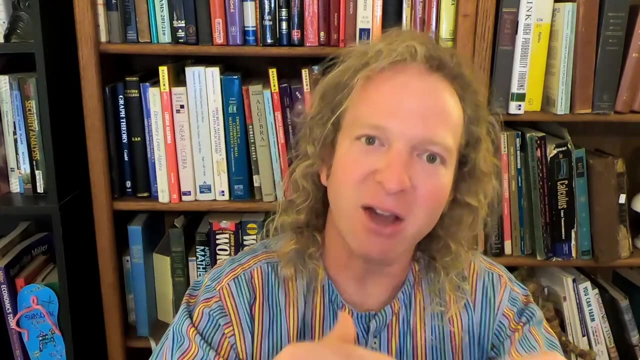 someone who has a proof and is a well-done proof, and emulate that right. you want to become better at writing proofs by watching other people write proofs and then creating your own from that, if that makes sense. so justify every step and that's how you learn how to justify your steps. it's by 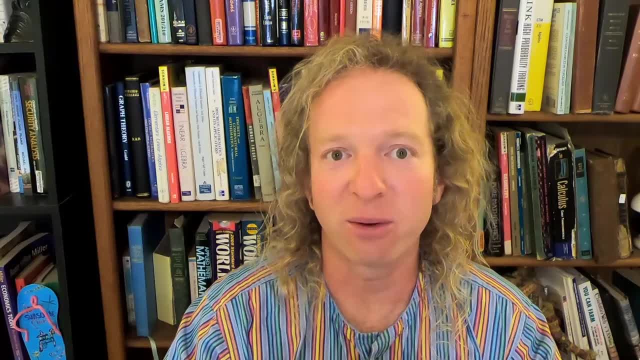 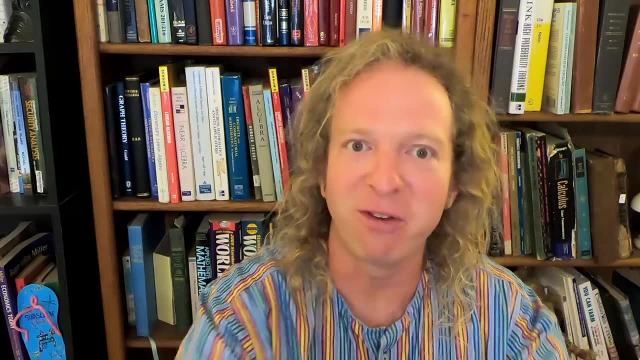 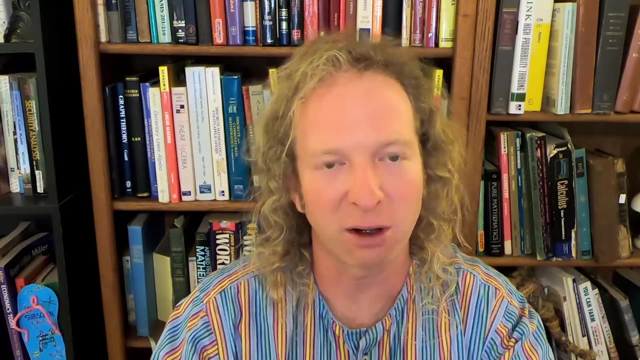 watching other people justify your steps. this is one of the occasions where i think videos are are extremely beneficial. uh, i don't mean, like you know, pump my own videos, but, uh, my abstract algebra videos and some of my advanced calculus videos and my topology videos, some of those, all my advanced 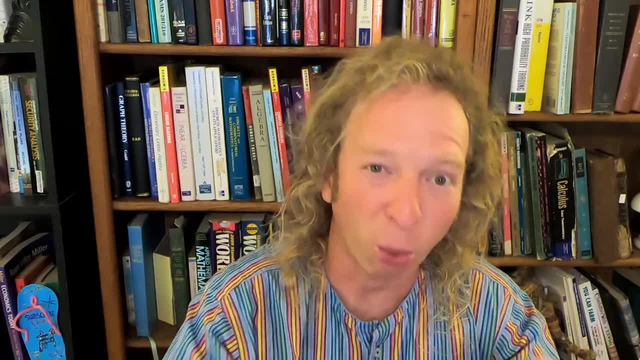 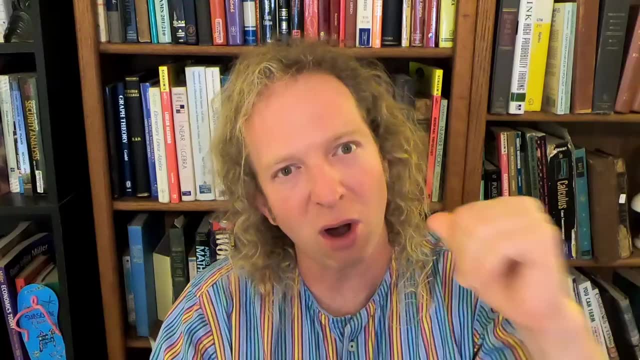 math videos. some of- not all of them, but some of them, in my view, are really, really detailed and good. not all of them are great. some of them are very good, but most of them are pretty detailed and they show all of the steps. so if you're taking a course like like abstract algebra, right. 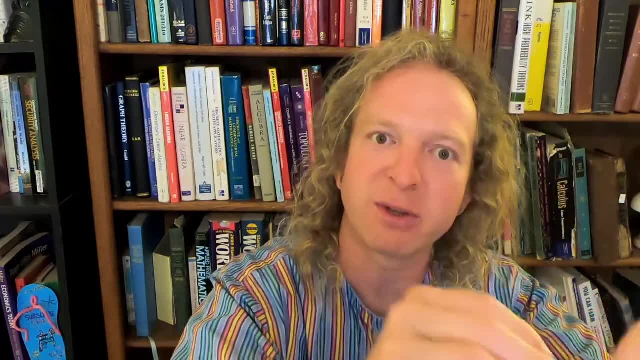 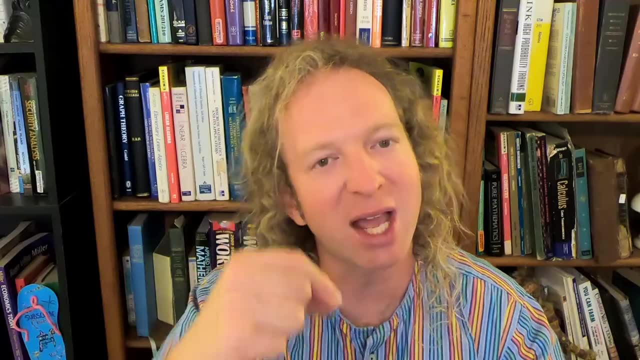 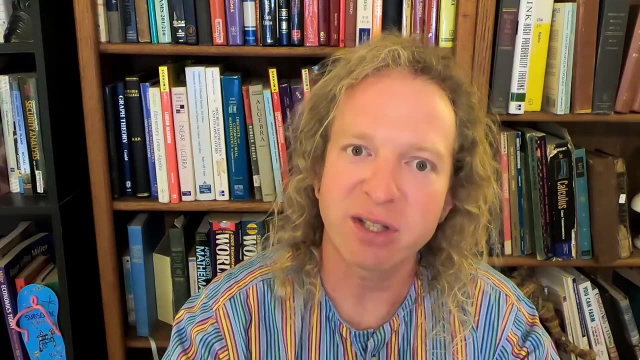 check out my videos right. go through my video and make sure you understand all of those steps and then try to redo those problems on your own and justify the steps. write down the why every single time. that's how you get better at writing proofs: by justifying every single step every single time, and that's how you'll know your. 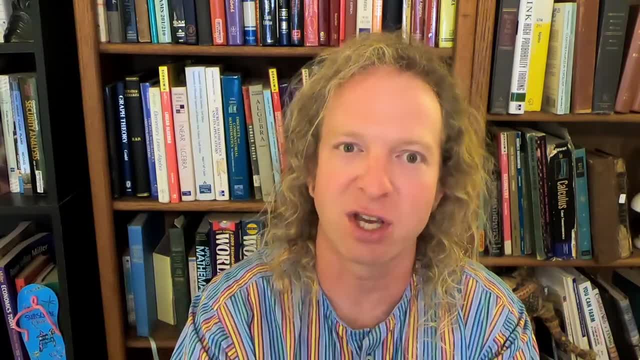 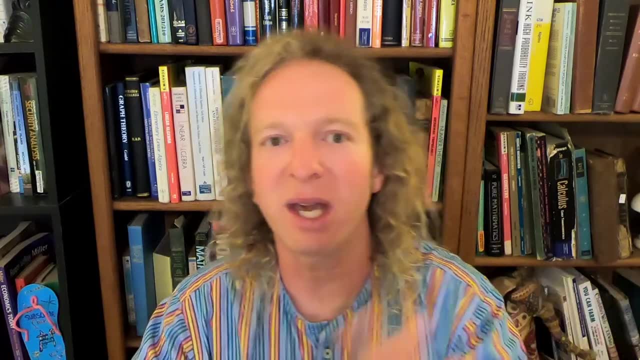 proofs are correct, because they're correct, because everything is justified. it's a big journey to learn to write proofs. in my view, it's one of the things that you get when you get your math degree. you know, you go to college, you get a four-year degree, you take all these classes and what do you?